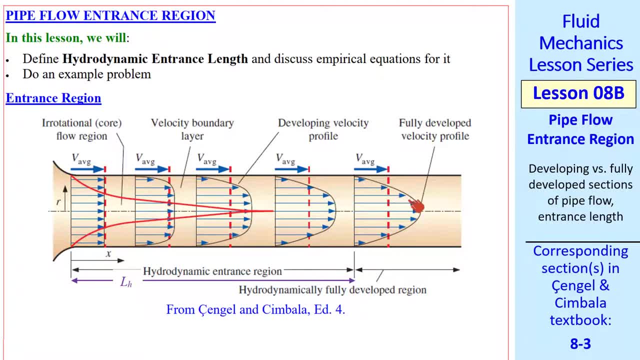 until eventually we get what we call fully developed. Fully developed velocity profile means that from here downstream this velocity profile no longer changes. There still is a pressure drop downstream because of friction on the wall. This is because of friction along the pipe walls. 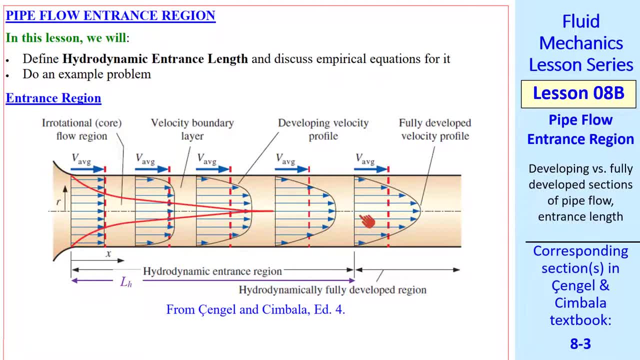 The region from the entrance to the location where it is fully developed is called the hydrodynamic entrance region. We use the adjective hydrodynamic because you can have other kinds of entrance regions, such as a thermal entrance region, which may be longer or shorter than the hydrodynamic entrance region. 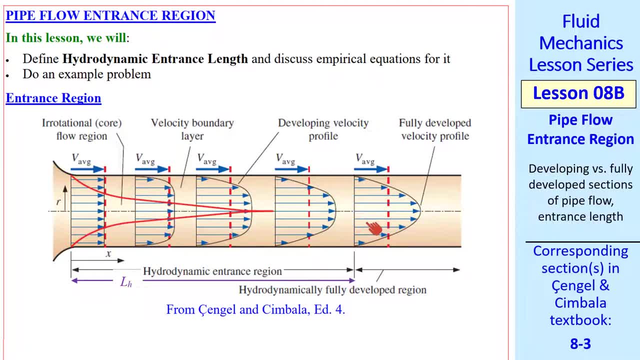 That would be the location where the temperature distribution becomes fully developed, which is not shown here. After the entrance region, we call this the hydrodynamically fully developed region. We'll talk about that in the next lesson. I wanted to point out qualitatively that the slope of this profile at the wall keeps changing within this hydrodynamic entrance region. 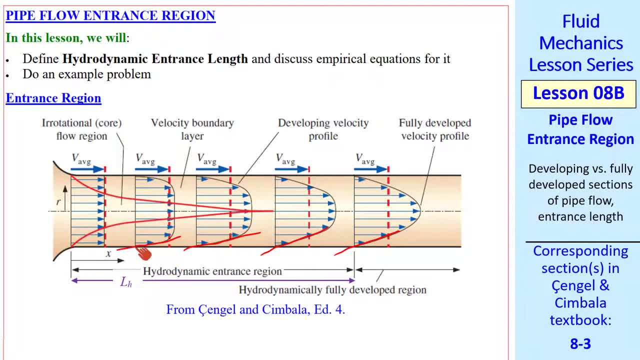 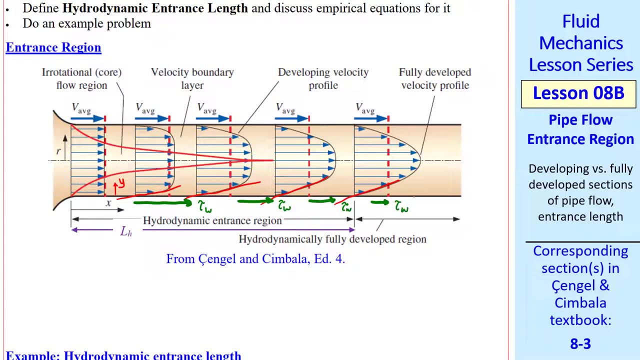 Since tau w, shear stress at the wall is proportional to the slope du dy, where we define y as the distance from the wall, you can see that du dy is decreasing as we go downstream, So shear stress, tau w, also decreases downstream. 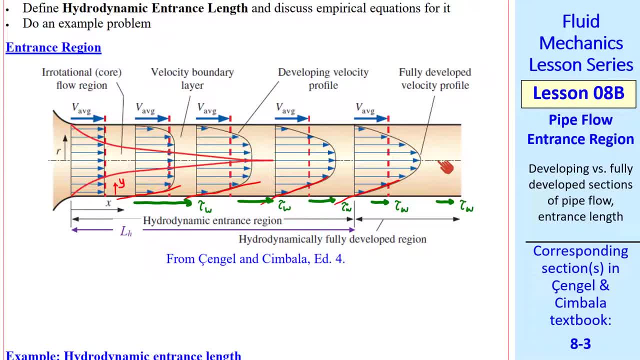 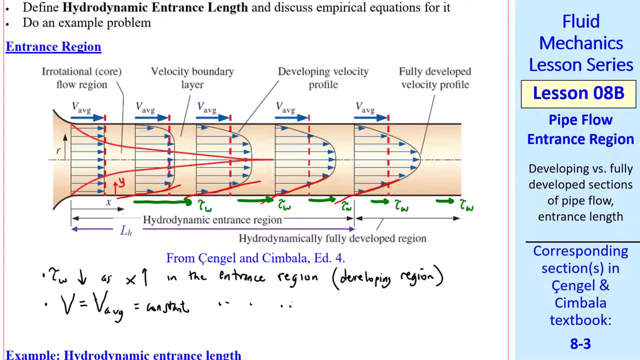 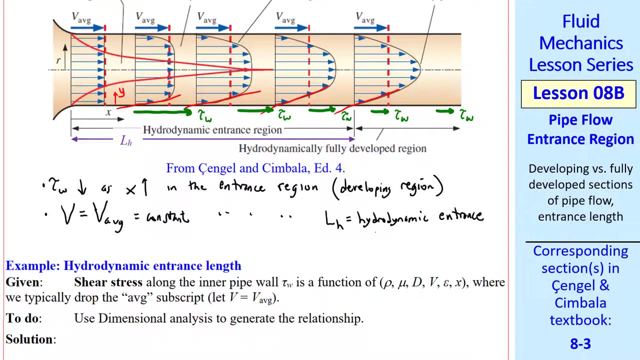 From then on it's constant in the fully developed region. So I write tau: w goes down as x goes up in the entrance region, also called the developing region. But v or v average is constant in the entrance region. You can see that here. Lh is the hydrodynamic entrance length. 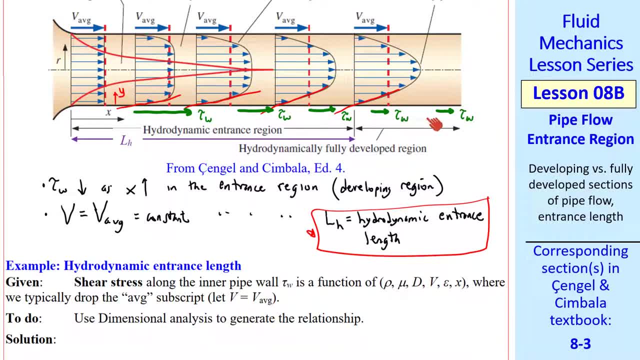 Because tau w is larger in the entrance region than it is in the fully developed region, this portion of the pipe has a higher head loss per unit length than does the fully developed region. In a later lesson we'll develop expressions to account for this entrance effect. 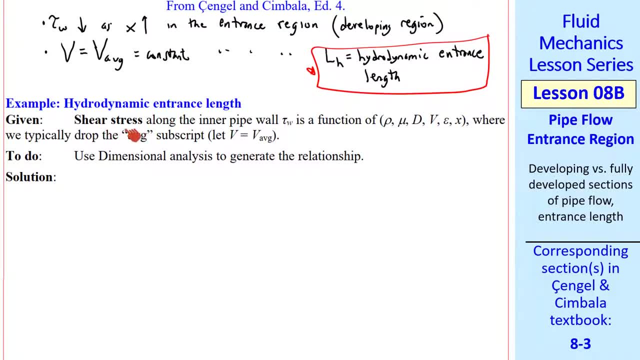 Let's do some analysis In this entrance region. the shear stress along the pipe wall is a function of rho, mu, d, v, epsilon and x, where we've dropped the average subscript, as we've done previously. v is the average speed through the pipe. 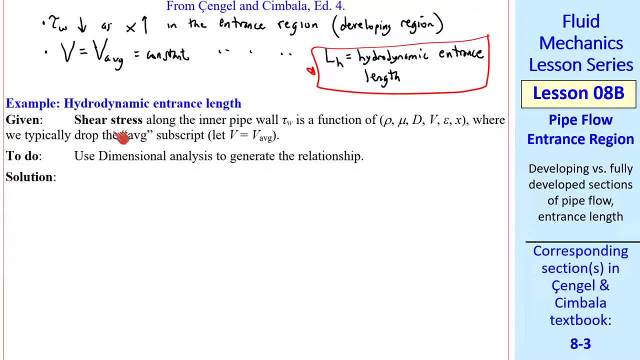 Let's use dimensional analysis to generate the relationship for shear stress. Recall from a previous lesson. we did this for fully developed pipe flow. We had tau, w as a function of rho, mu, d, v and epsilon, And dimensional analysis yielded the dependent. pi was f, the Darcy friction factor. 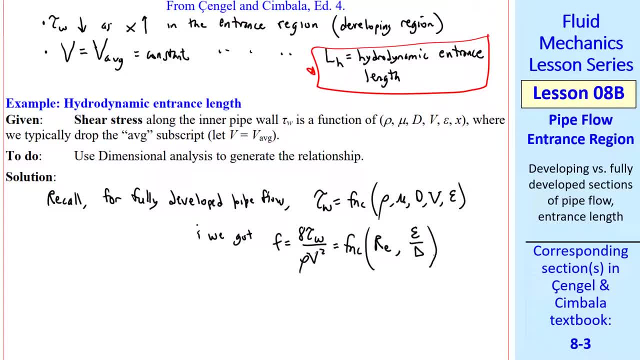 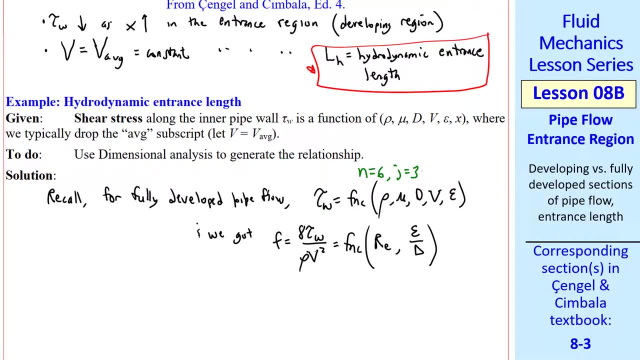 is a function of Reynolds number and relative roughness, epsilon over d. In this case we had n equals 6, the number of variables j equals 3, the number of repeating variables. therefore, k equals 3 pi's. Now we add x to our list of independent variables. 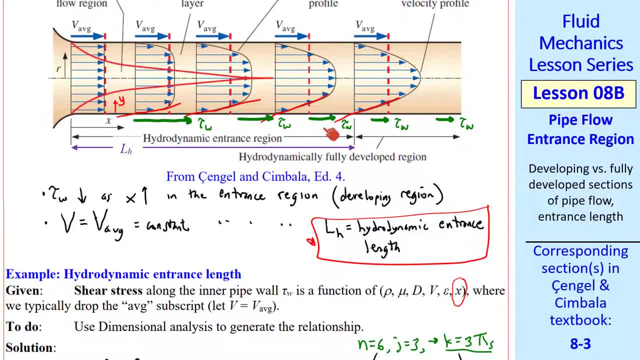 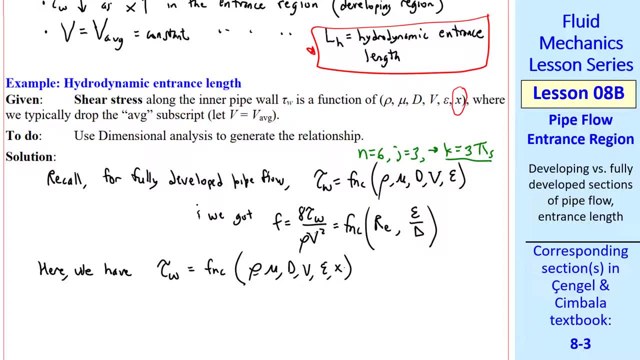 Since tau w for the entrance region is constant. in the entrance region the entrance length depends on x, as I've shown here. So here we have: tau w is a function of rho, mu, d, v, epsilon and x. So n equals 7, j is still 3, so we expect 4 pi's. 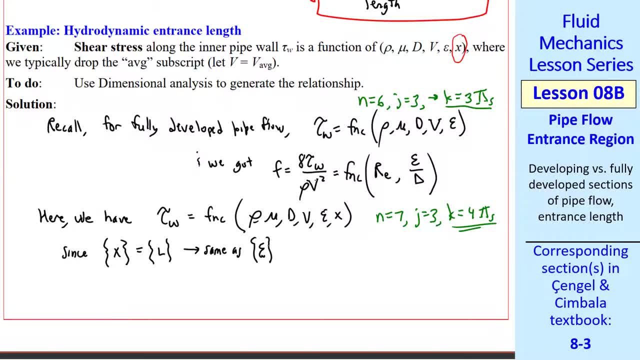 We can do this one in our head. Since the dimensions of x are length, which is the same as epsilon, the roughness, we expect our fourth, pi, to be the same form. So, instead of that expression for fully developed pipe flow for the entrance region, 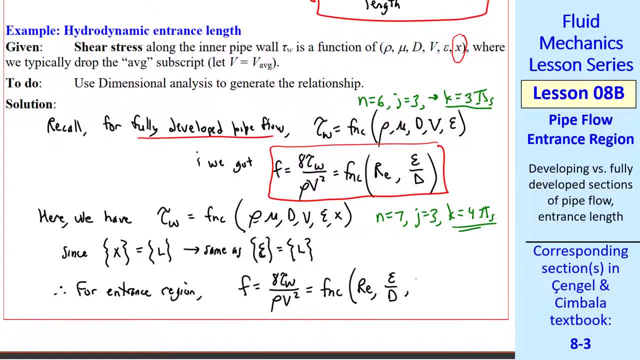 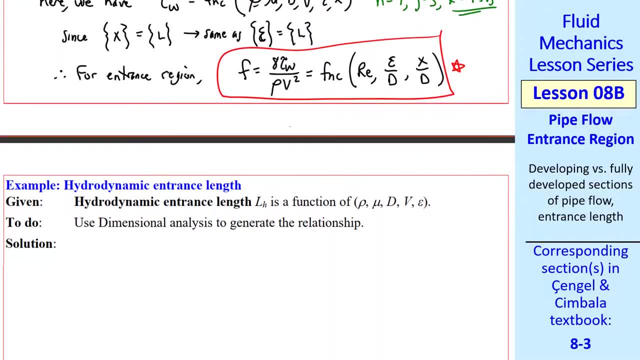 the friction factor is now a function of Reynolds number, relative roughness and x over d. You're welcome to try this one on your own from scratch, for practice. Let's do a similar analysis for the actual entrance length. Lh is a function of rho, mu, d, v and epsilon. 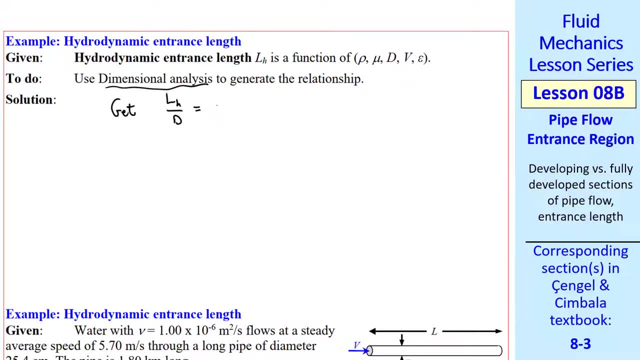 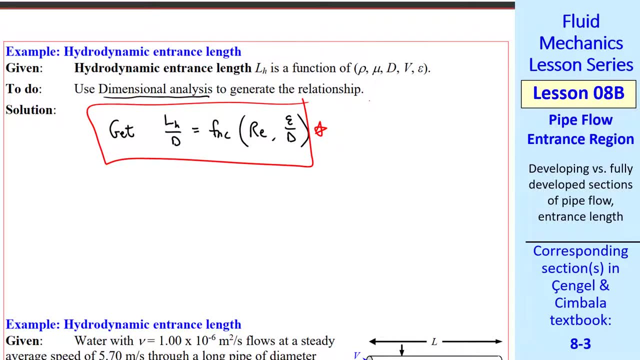 We use dimensional analysis again. I'll just give you the result. You can try this one on your own for more practice. You may not be surprised at this answer, since it's very similar to the previous problem where Reynolds number is rho v d over mu. 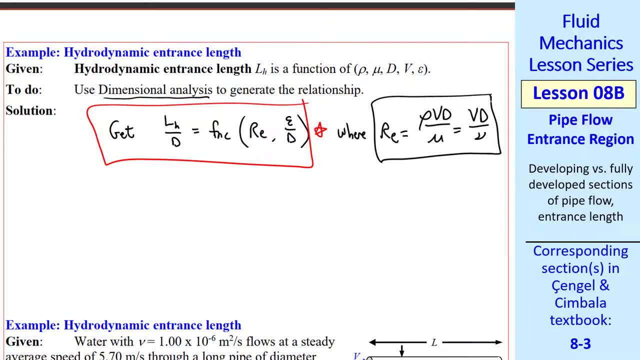 or v d over nu, since nu is mu over rho, It turns out in practice epsilon has little effect on Lh. So if we let Lh over d be a function of Reynolds number only, it's a reasonable approximation. 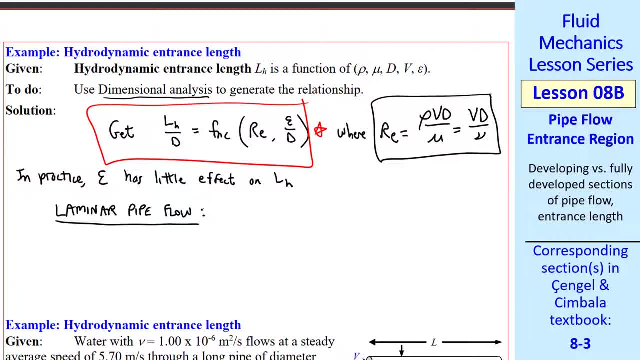 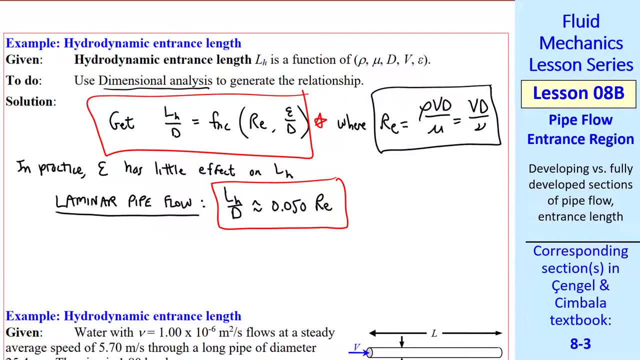 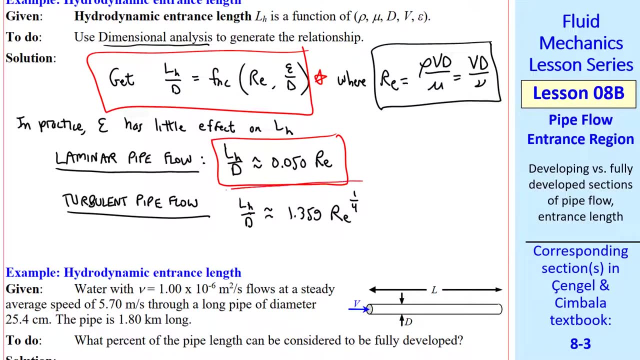 Here are some experimental correlations or empirical equations. The entrance length parameter Lh over d turns out to be 0.050 Reynolds number. Note that this is approximate For turbulent pipe flow. it turns out that Lh over d is approximately 1.359 times Reynolds number to the one-fourth power. 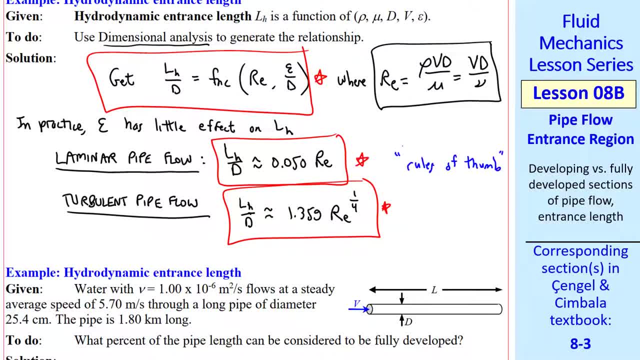 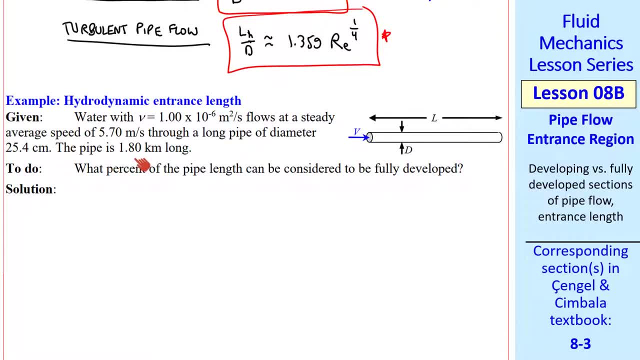 These are rules of thumb or ballpark estimates for entrance length. Now let's do an example. Water flows at a steady average speed through a long pipe with a given diameter and length. We'll assume we have a nice, well-rounded inlet. 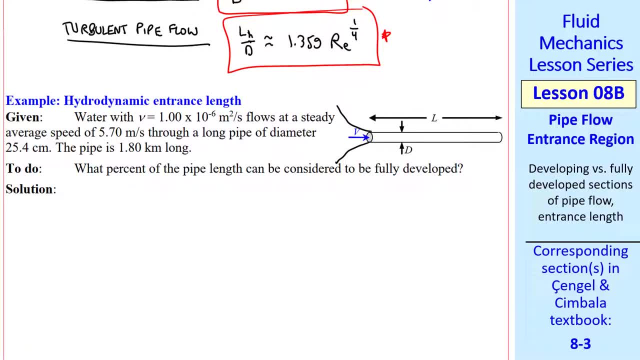 so that we have an entrance region like we sketched previously, And the entrance length will be some portion of this pipe length. We're asked to find the percent of the pipe length that can be considered fully developed, That would be this portion downstream of the entrance length. 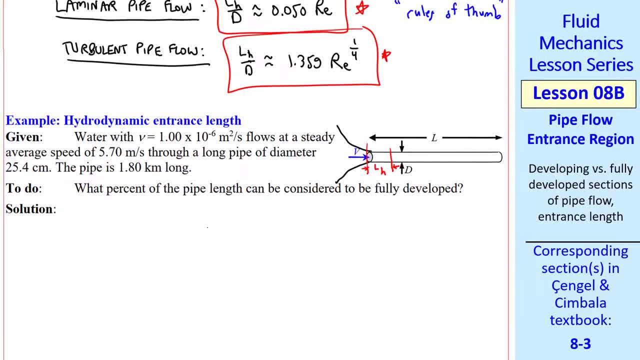 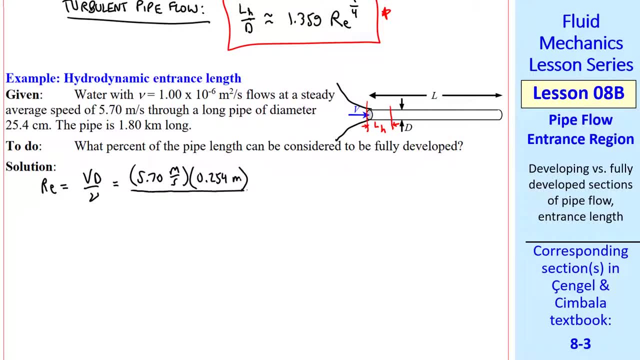 Well, first we must determine whether this flow is laminar or turbulent. So we calculate the Reynolds number Re equal Vd over nu, We plug in the given values, being careful with units as always, And we get about 1.44 million as our Reynolds number. 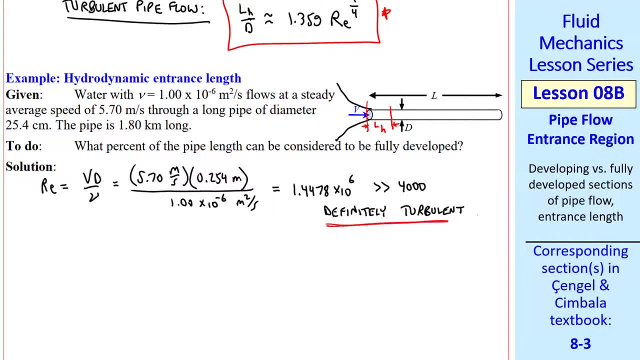 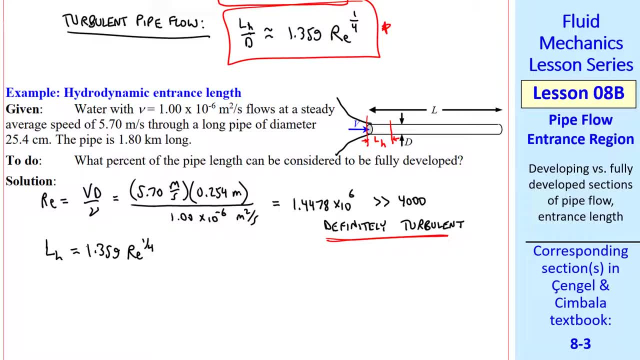 This is much greater than 4000. So this flow is definitely turbulent, And thus we use this empirical equation. We write it as Lh equal 1.359 Reynolds number to the fourth times d, We plug in our Reynolds number and our diameter. 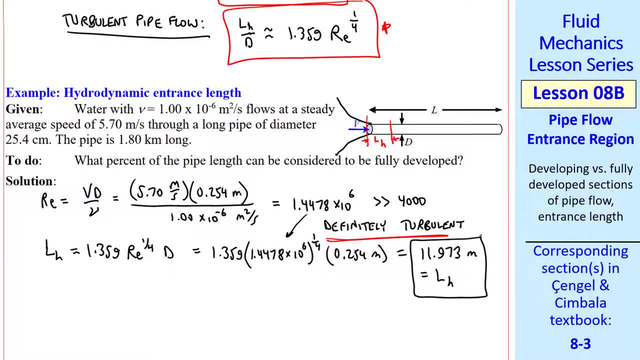 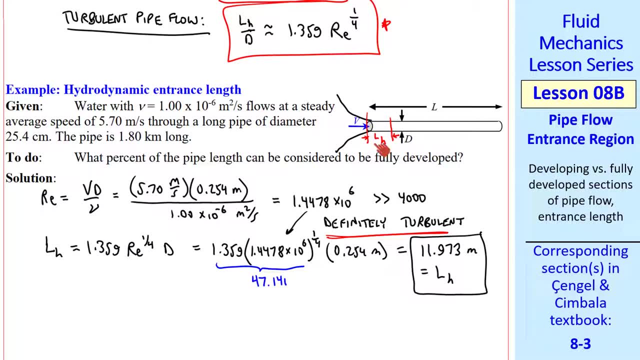 And we get: Lh is 11.973 meters. By the way, this quantity turns out to be 47.141, which is Lh over d in this equation. In other words, the entrance length is approximately 47 pipe diameters. 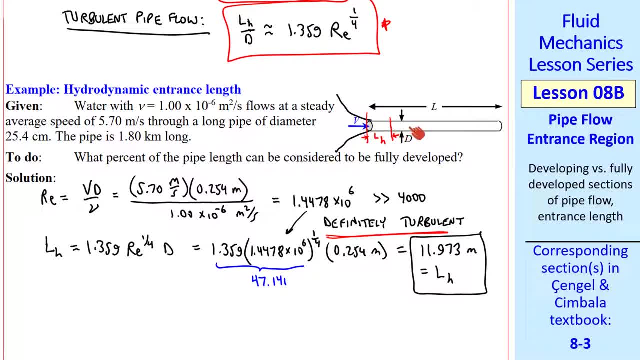 That's how long it takes for this flow to become fully developed. But the actual pipe is very long- 1.8 kilometers. So the percent of the pipe length that can be considered to be fully developed is calculated as L minus Lh. 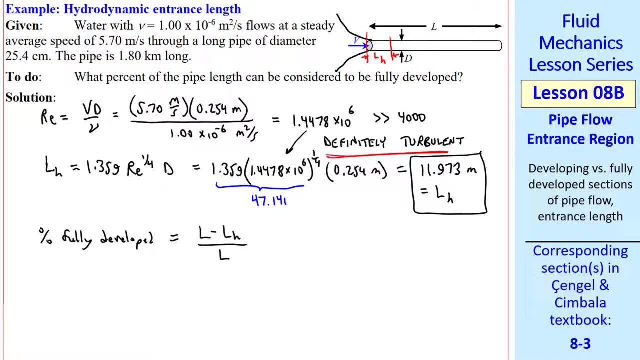 That's this section of the pipe divided by L, which is the whole pipe length times 100%. since we're asked for a percentage, This part is fully developed And this is the total pipe length. Plugging in our numbers and having consistent units, 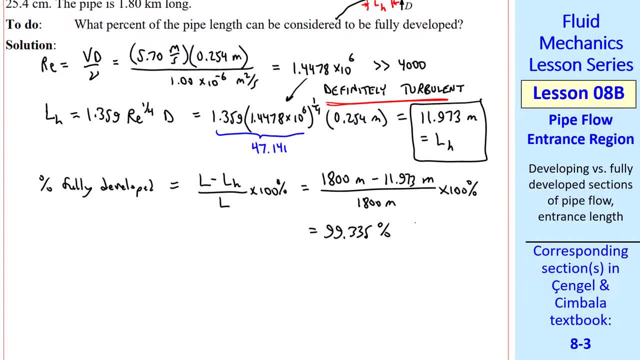 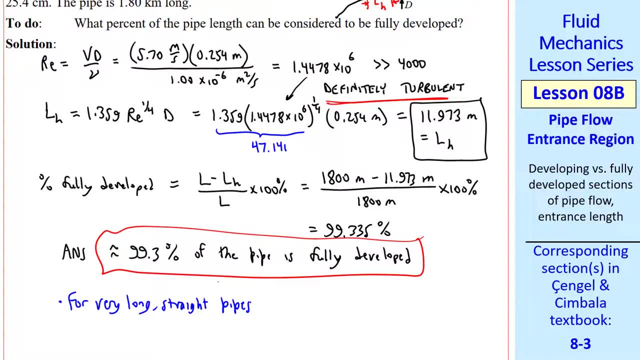 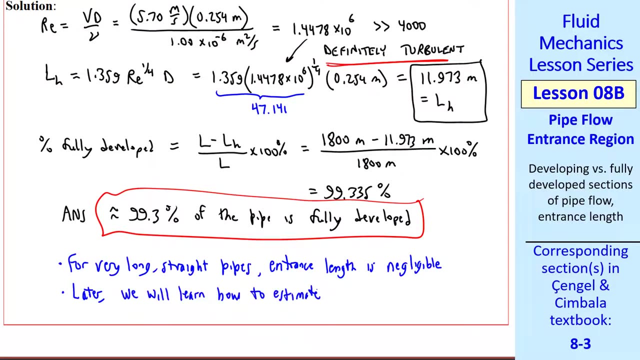 we get 99.335%. So our answer is that 99.3% of this pipe is fully developed. You can see that for very long straight pipes, such as a water pipe like this, entrance length is negligible or insignificant. In a later lesson we'll learn how to estimate.